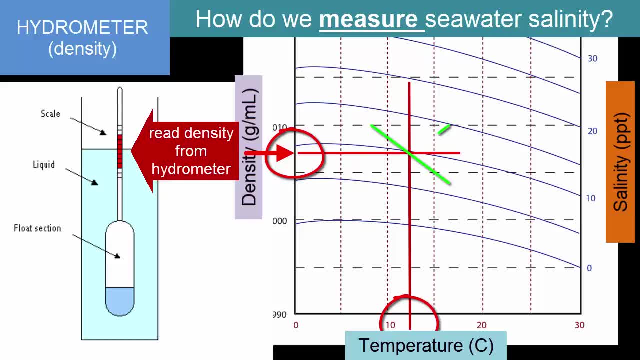 Measure density, pick the line that represents the right temperature and, from that, determine salinity. Again, like the salinometer, this works only because we already know the main constituents of seawater and their constant proportions. That allows us to calculate these lines and draw these graphs based on the known weights. 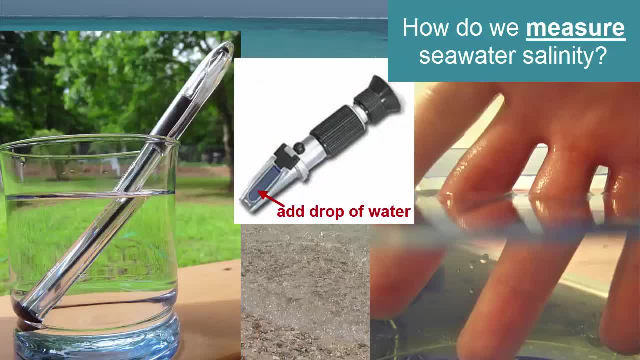 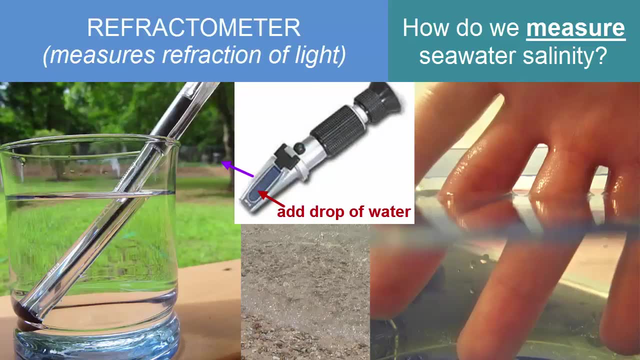 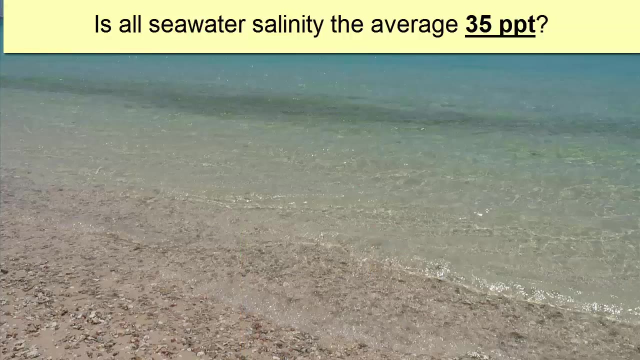 and proportions. Another method for measuring salinity is the refractometer, which measures the angle at which light bends or refracts, a property that changes as salinity changes. Though the oceans have an average salinity of 35 parts per thousand, there are local 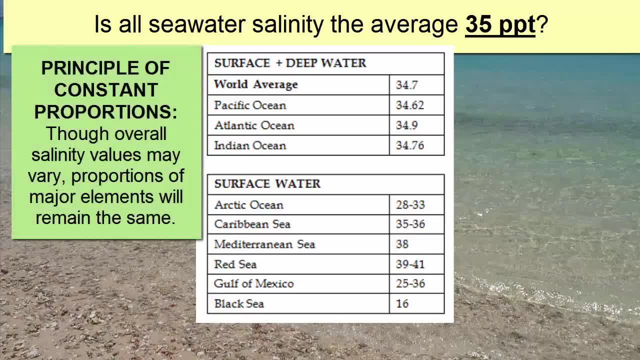 variations. Remember: the proportions of the dissolved ions stay the same, but the total amount can vary. What are some of the major processes that affect salinity of the water? What are some of the major processes that affect salinity of the water? What are some of the major processes that affect salinity of the water? 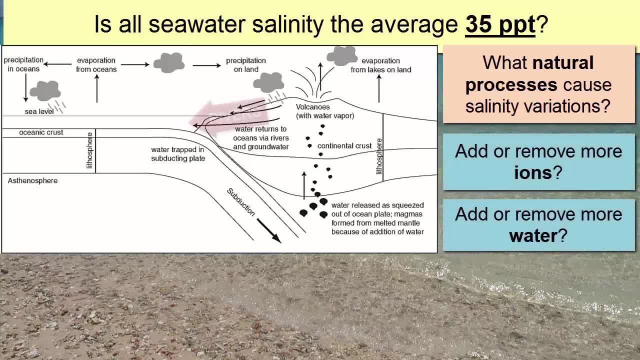 Do we want to break down these local variations of oxygen indexing into light colour? Why are MCOs possible in the natural water and create these local variations? what are some of the major processes that affect salinity of water and create these local variations? 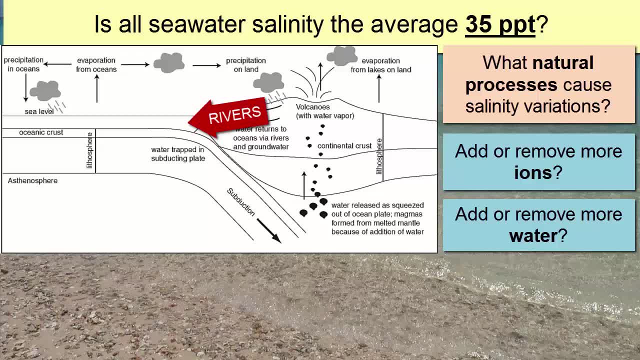 Since the major source of these ions is river water, but only over billions of years of collecting, we can't simply add more ions quickly to create a local variation. So, since we can't add or remove ions quickly, we will have to focus on changing salinity. 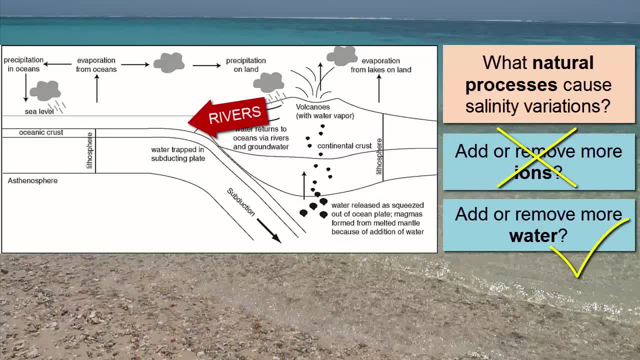 by adding or moving water. So since we can't add or remove ions quickly, we will have to focus on changing salinity by adding or removing water. If we can add more fresh water to an area of the ocean, there will be a local reduction. 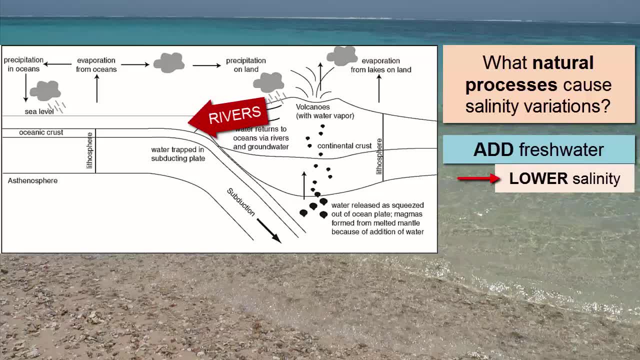 in salinity there. So if I follow that chart- and this is thebey that I use to estimate the angle of salinity there, as that fresh water slowly mixes, Similarly if we can remove fresh water, there will be a local increase in salinity. So what are the natural methods? 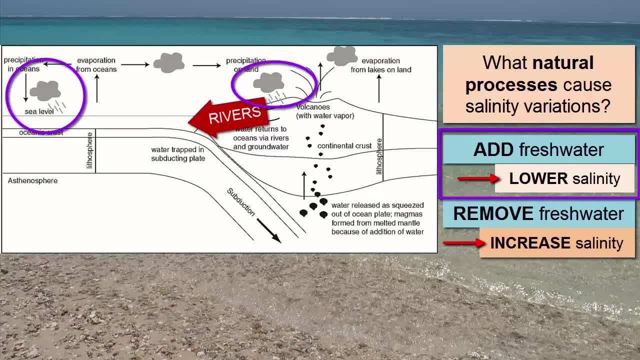 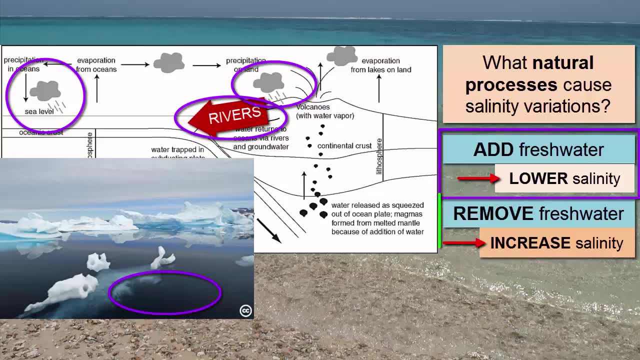 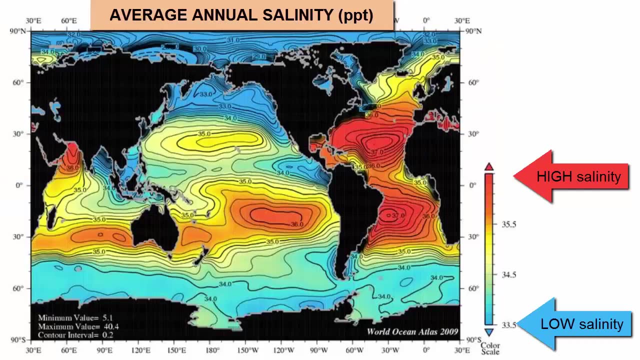 for adding or removing fresh water. For adding water, there is rain, precipitation, runoff, river mouths and melting ice. For removing water, there's the opposite: formation of sea ice and evaporation. Now let's look at a map showing the average surface salinity of the entire world ocean, The freshest.